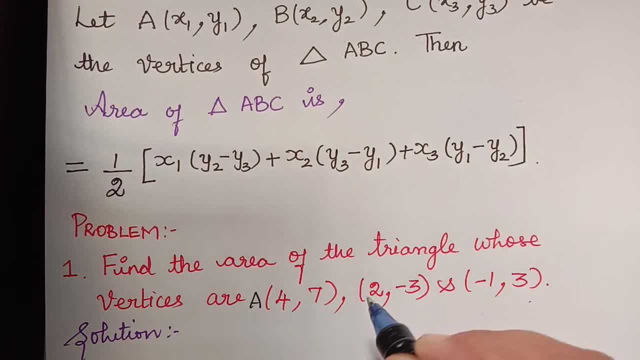 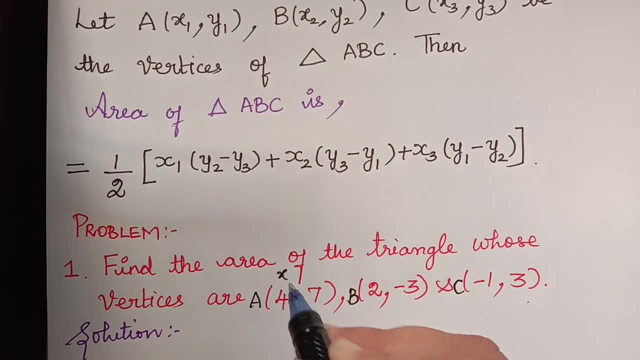 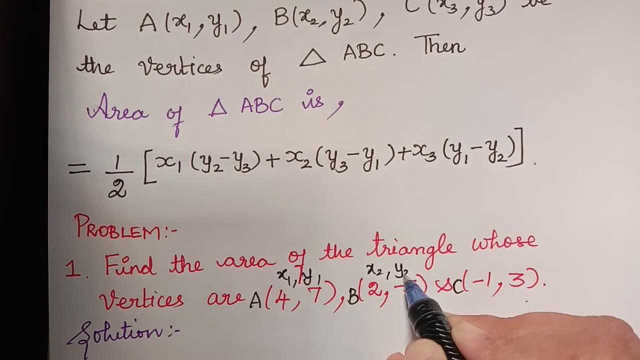 name these vertices. Let this be vertex A and this is B and this is C. So this coordinate of A will be x1 comma y1 and this will be x2 comma y2 and this is x3 comma y3.. So these are the values of. 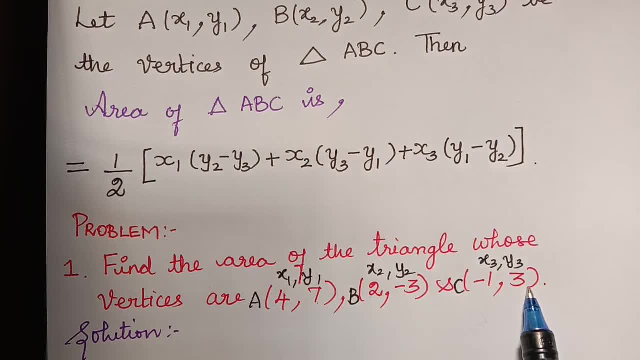 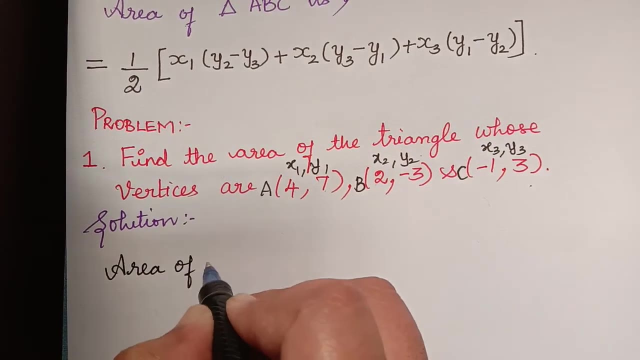 x1, y1, x2, y2, x3, y3.. Now let us substitute these values in this formula and we will find the area of the triangle A B, C. So therefore, the area of triangle A B C. 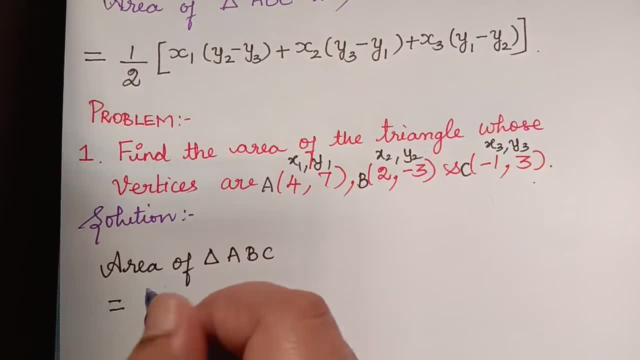 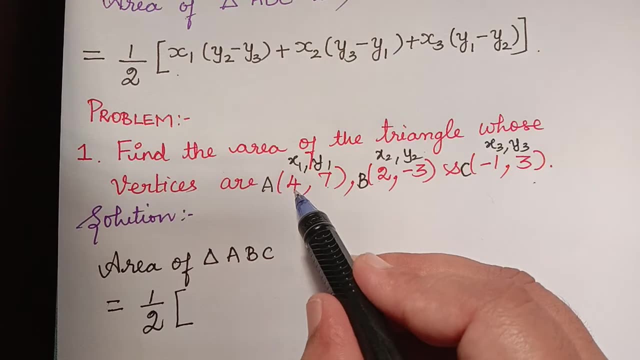 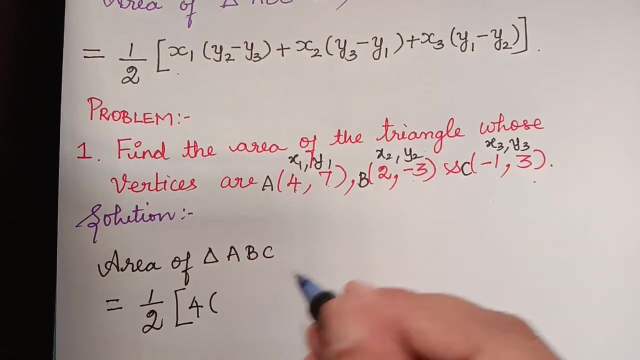 will be equal to- so I will write it here- 1 by 2 of x1.. So what is x1? 4. So 4 multiplied with y2 minus y3. So y2 is minus 3 minus y3. So minus. So here we have a plus sign. So it will be minus 3 and then plus. 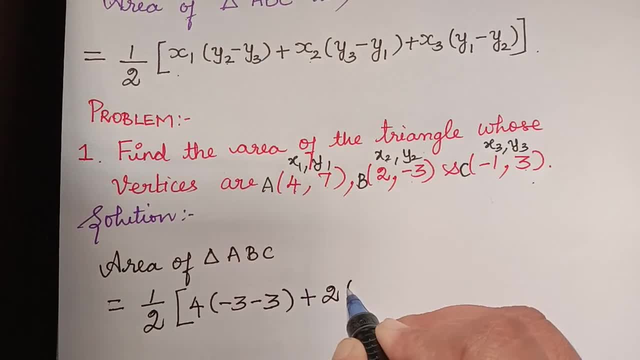 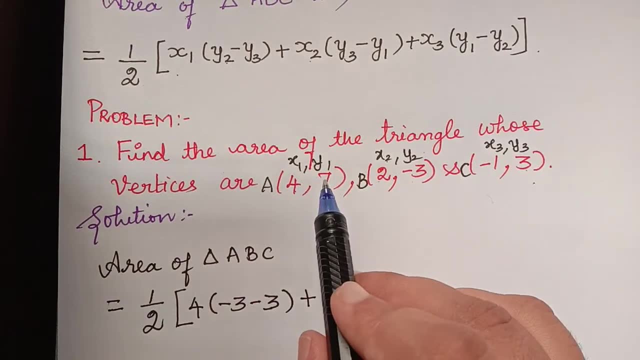 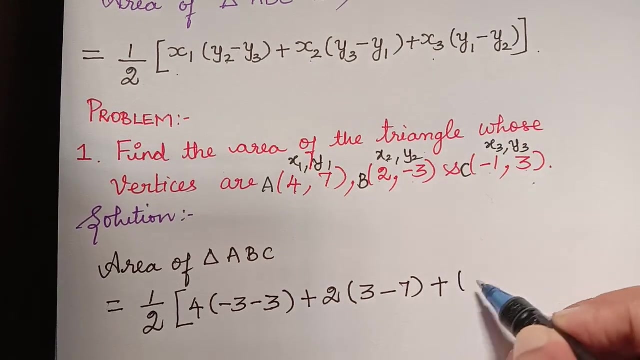 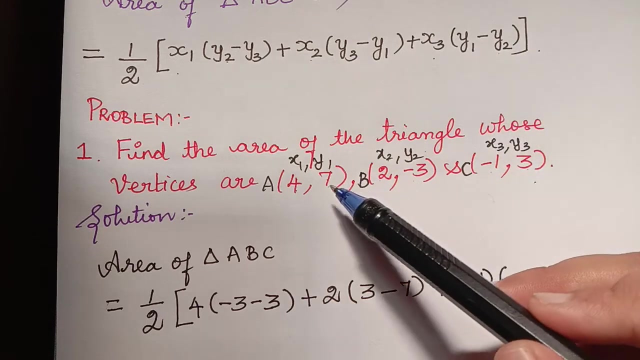 2.. So x2 is what 2 multiplied with y3 minus y1.. y3 is 3 minus y1 is 7 plus x3.. What is x3? Minus 1.. So minus 1 multiplied with y1 minus y2.. What is y1? y1 is 7 minus y2 is minus 3.. 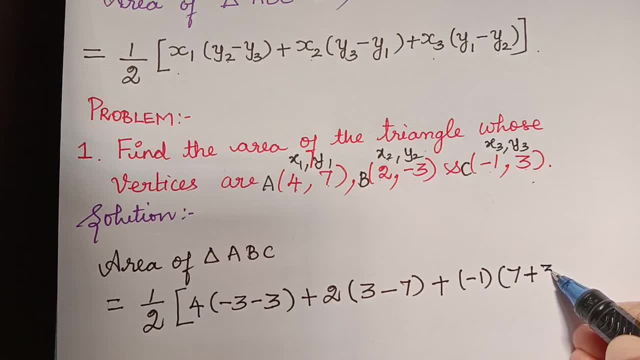 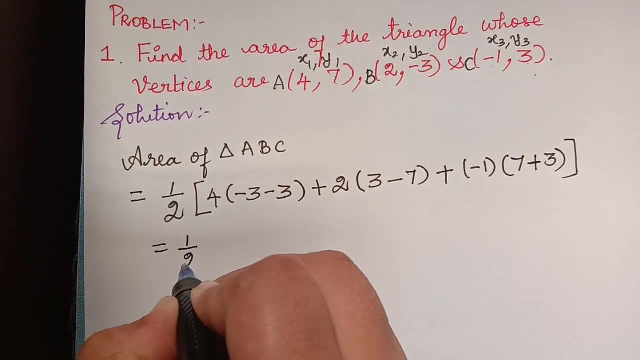 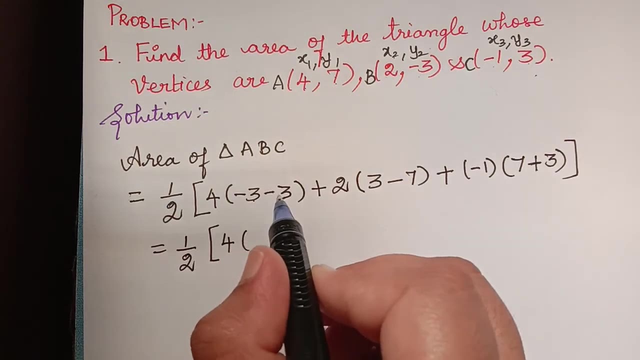 So minus of minus 3 will be plus 3.. So let us simplify this now, So that will be equal to 1 by 2 multiplied with 4, multiplied with what is minus 3, minus 3.. So negative 3, negative 3 we have to add. 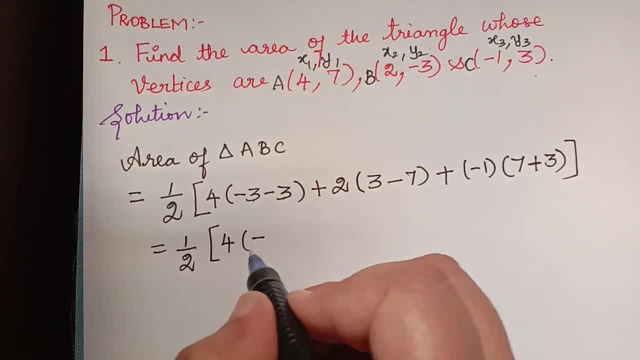 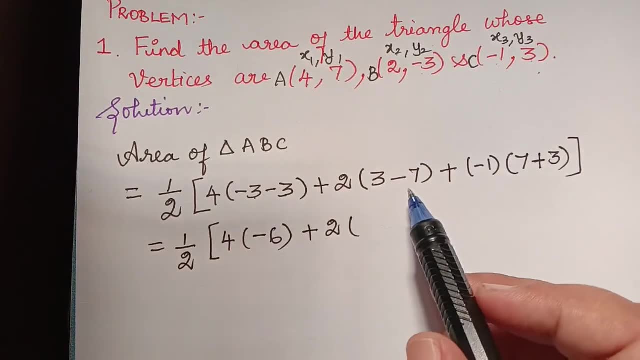 both, It will be negative 6 and we have to give the negative sign. So negative 6 plus 2 multiplied with 7. we have to subtract these two, So it will be 4 and the highest number sign is minus. So 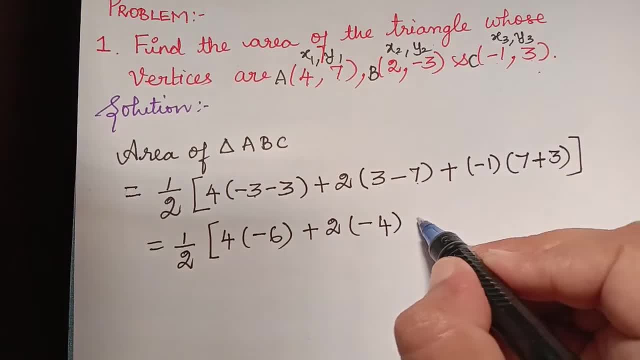 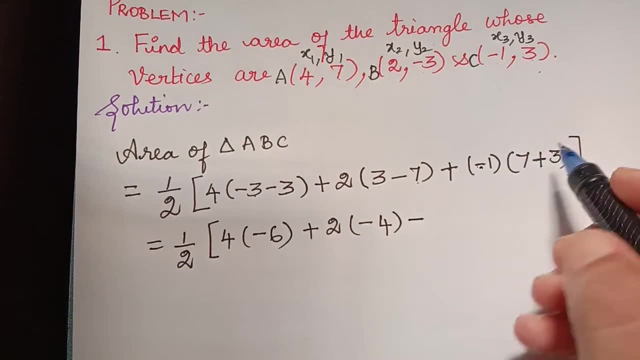 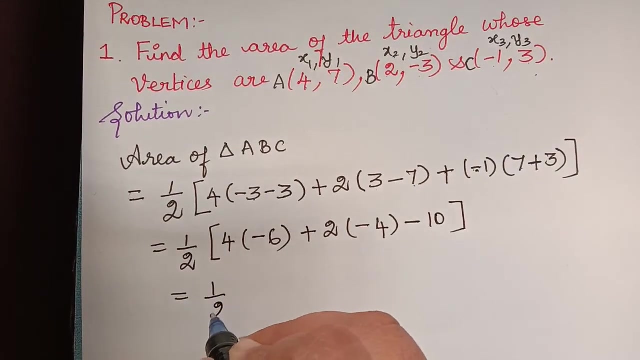 we will be having minus 4 and here we have a negative sign. So plus multiplied with this negative, it will be minus. and what is 7 plus 3?? It is 10, and simplifying this further, this will be equal to 1 by 2 of. let us multiply these two. 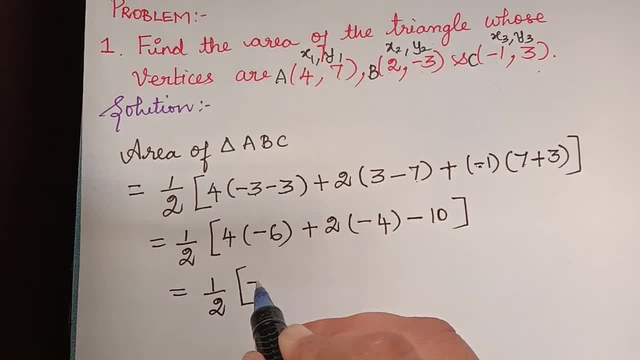 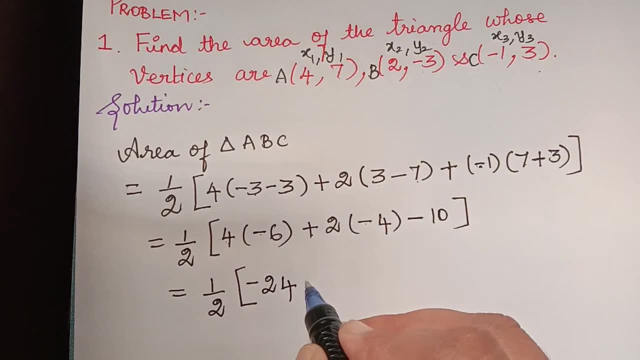 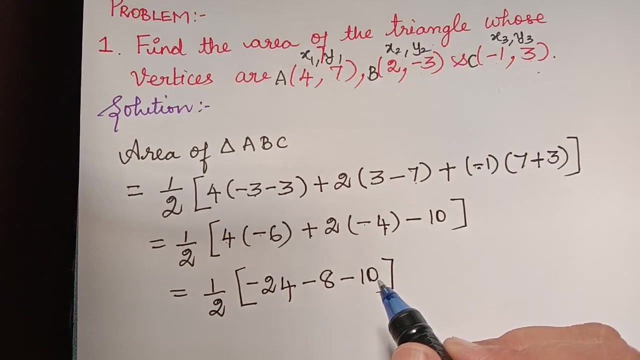 So 4, 6 times is 24.. So it will be a plus into minus. So minus 24 and plus multiplied with minus will be minus 2. multiplied with 4 is 8 and minus 10.. So now we have to simplify this further. 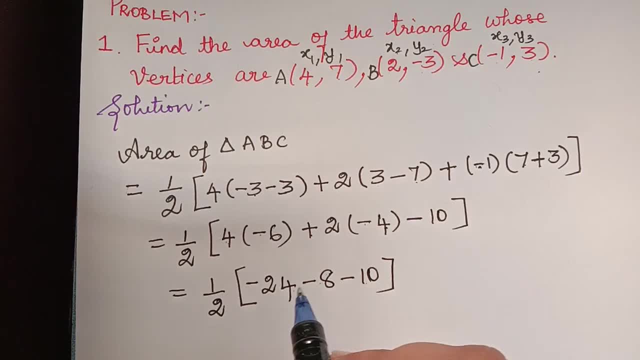 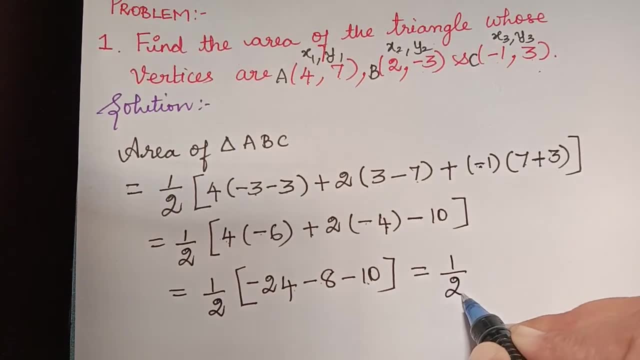 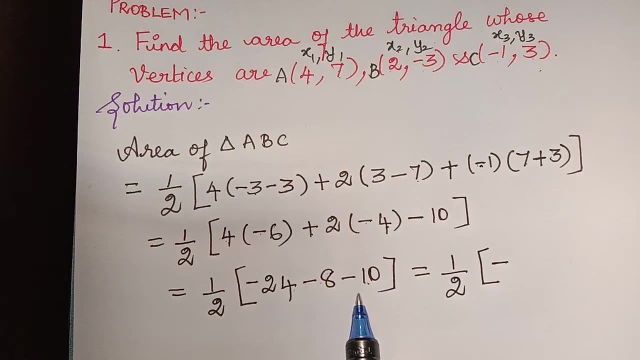 So all are having negative sign. So we have to add all the three and we have to write a negative sign in the front. So this will be equal to 1 by 2.. So 24 plus 8 plus 10 is what we have to do, And that will be 42. And so it will be negative 42. 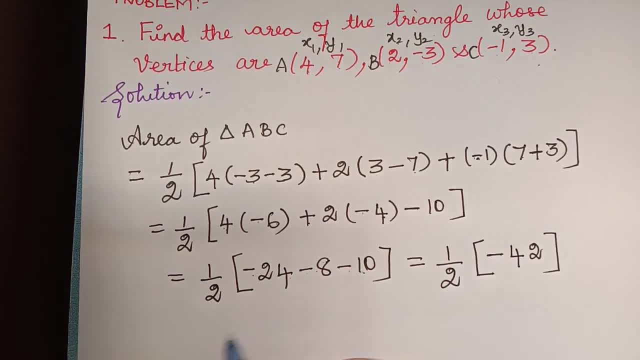 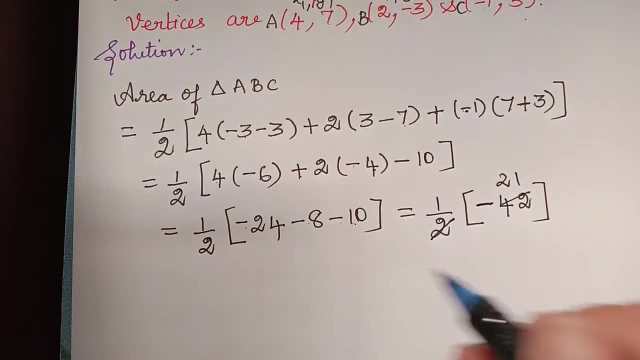 as we are having negative sign throughout, And so this gets cancelled and we get 21.. And we have a negative sign here and therefore the area of the triangle ABC is equal to negative 4 plus 5.. And so we have to do, and therefore these two will be equal to. 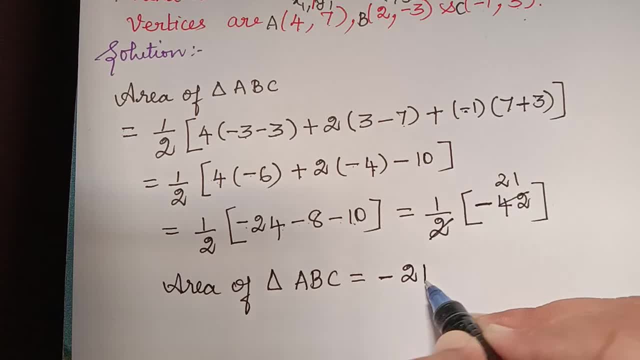 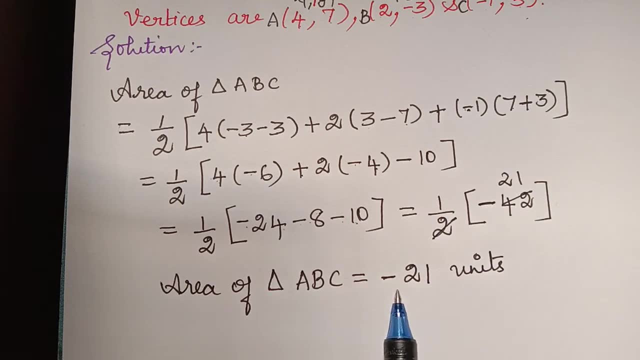 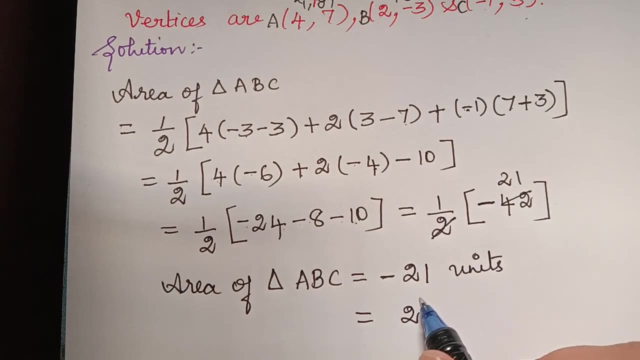 to negative 21 units. but we know that area we need not mention as a negative quantity. we have to be so therefore we can write this as just 21 and this is, this is area. so area is obviously square units, it will be square units. so therefore the solution of the given problem is: 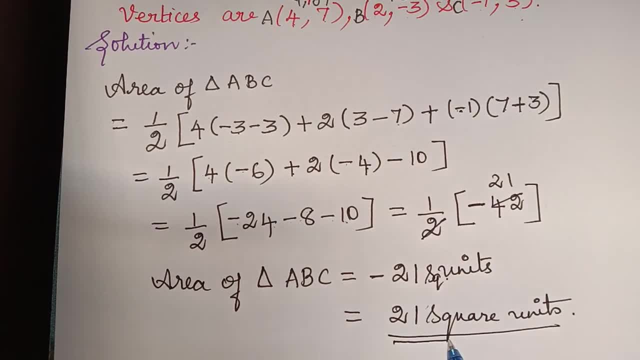 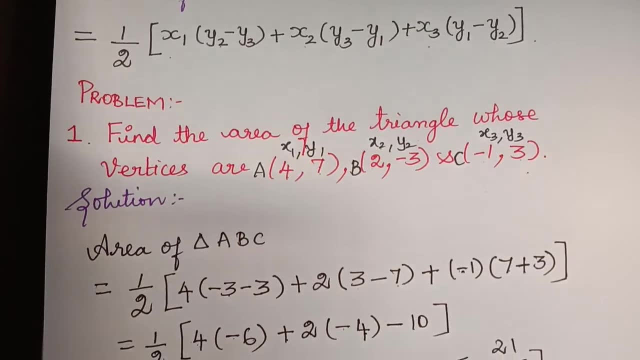 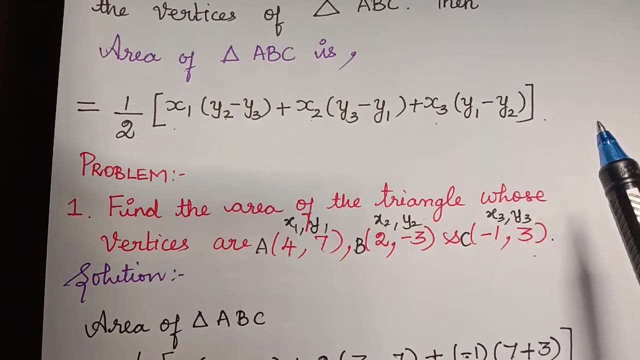 21 square units. hope you have understood how to find the area of a triangle. I would like to add a note here. that is, if we want to prove that three points are collinear. so what is collinear? the area of the triangle is 21 square units, so the area of the triangle is 21 square units.